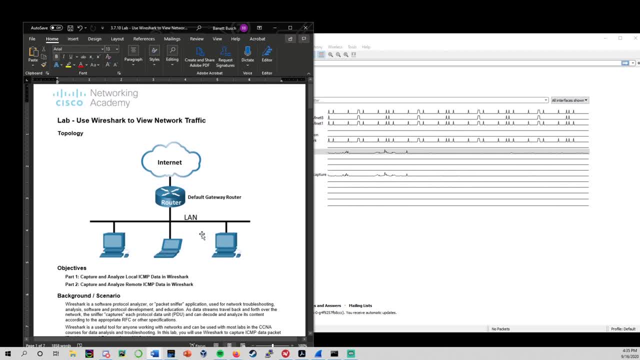 Network traffic, both on our internal systems, and then also we're going to capture traffic that we're connecting to remotely or out on the internet, essentially remote hosts. So we'll be working with ICMP, ping requests And the first part of the lab. we're thinking only internally. 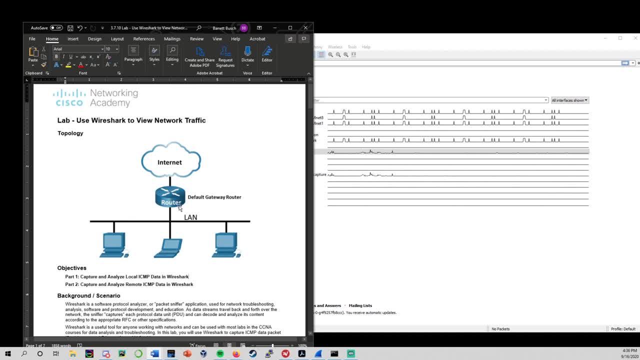 Only local data In part two of the lab. that's when we're going to start. We're going to ping outside websites like googlecom, ciscocom and, I believe, yahoocom. So you may be thinking: okay, what is Wireshark? 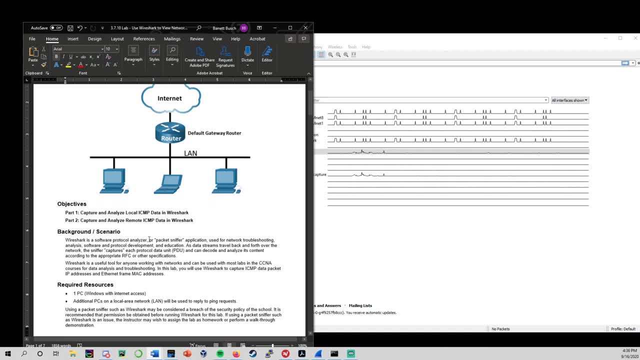 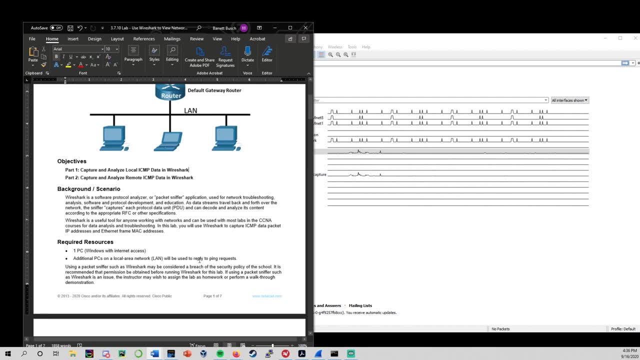 What is packet sniffing? So in this scenario here it describes it all really well. Wireshark is a software protocol analyzer or packet sniffer. It's used for network troubleshooting, analysis, software and protocol development and, as we're doing right here, for education, right. 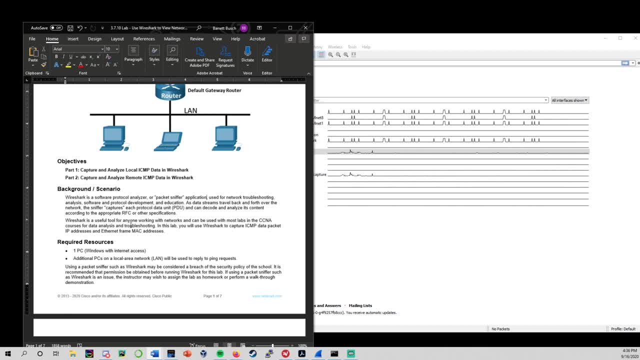 So we're using this to get a detailed look at what happens when you make a ping request and how this data transfers between networks. As data streams travel back and forth over the network, the sniffer captures each protocol data, So this is the data that's being processed by a unit or PDU and can decode and analyze its content according to the appropriate RFC or other specifications. 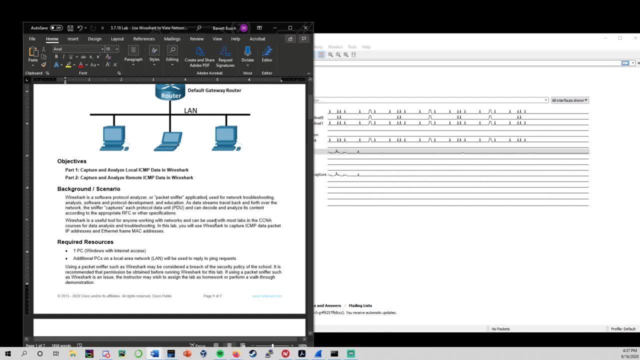 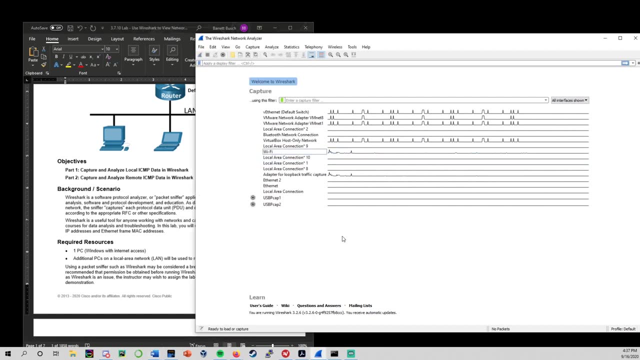 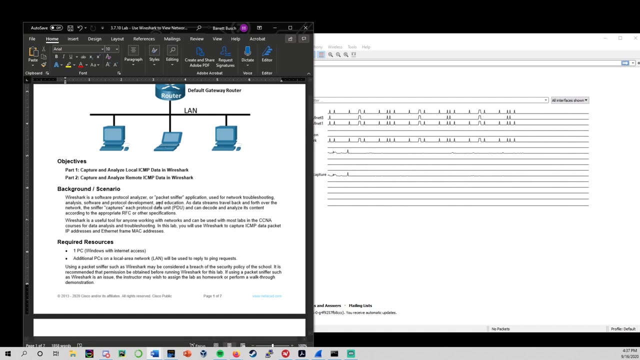 So these captures you know, you'll probably remember from the sample quiz for this week, We looked at what were called PCAP files. That is essentially a Wireshark capture that was kind of frozen in time from the moment All of those packets were captured and we were able to analyze that. 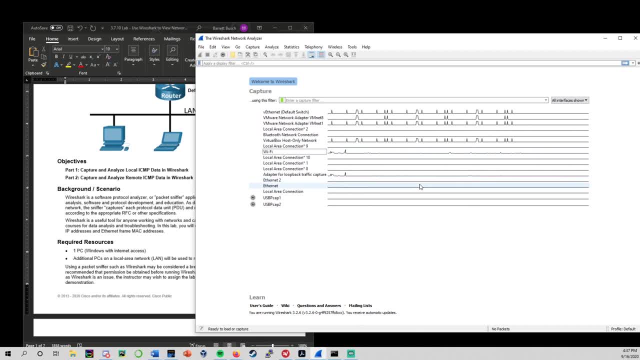 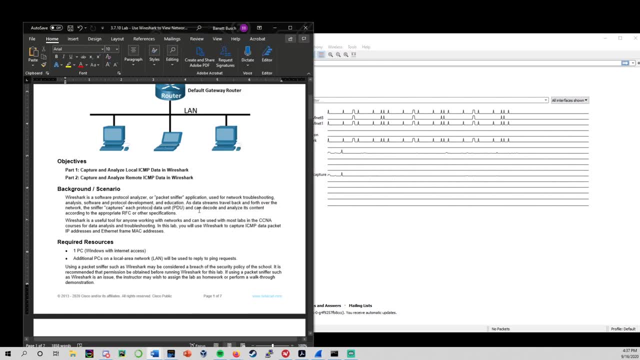 So that's essentially what we're doing. We're going to capture real-time network traffic happening on your own network at home and then we'll be able to look at those ping requests that we make. So required resources: you just need essentially just your one PC. 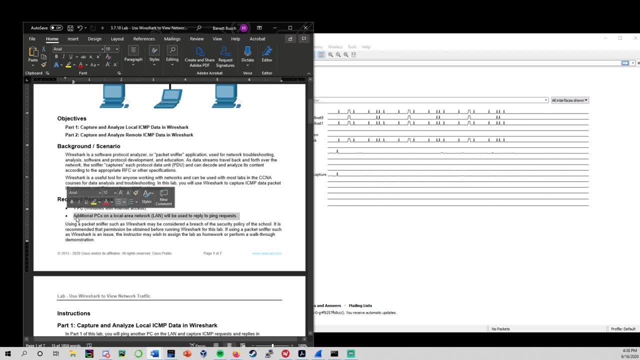 Now, this was back when this was done on campus. You had a teammate in your classroom and each person's computer obviously had its own separate internal IP address. So it was really nice to work with a partner on this, But you can do this at home as well. 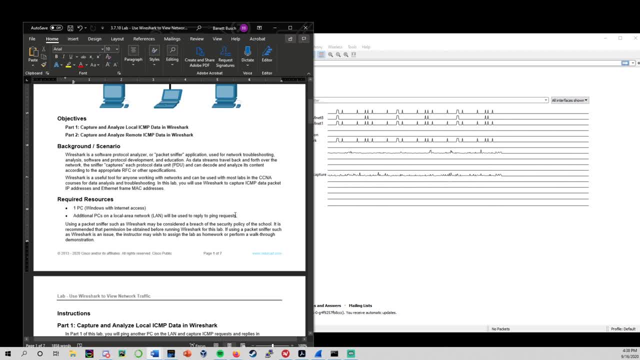 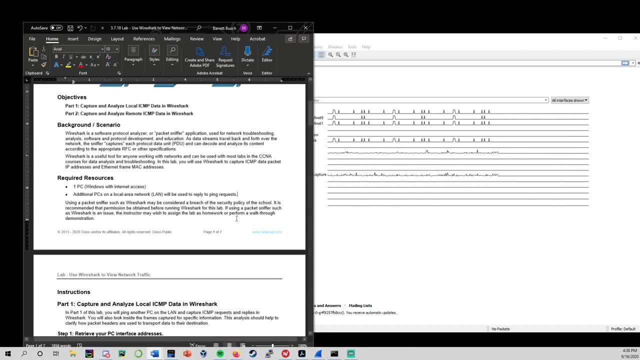 You could potentially, if you maybe have a desktop PC and you have a laptop, you could get the IP address of your laptop as well and you could ping back and forth between those two. But in the video- In the video I'm going to do what a lot of you may also want to do and you could. 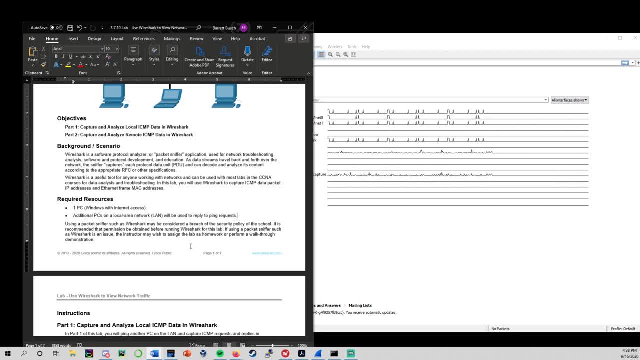 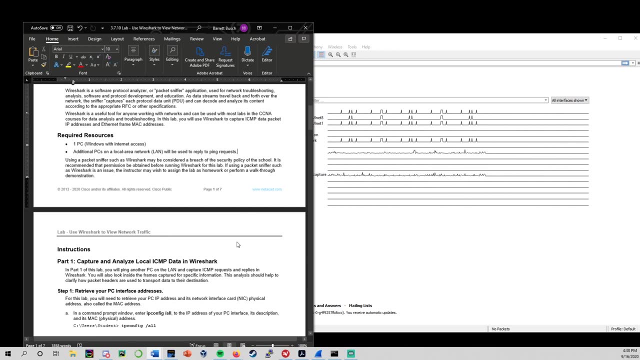 just ping your default gateway or your router and I will show you in a little bit how to get that information, how to get that IP and also MAC address. So since we're all doing this at home, I'll use that as the main example, since that will. 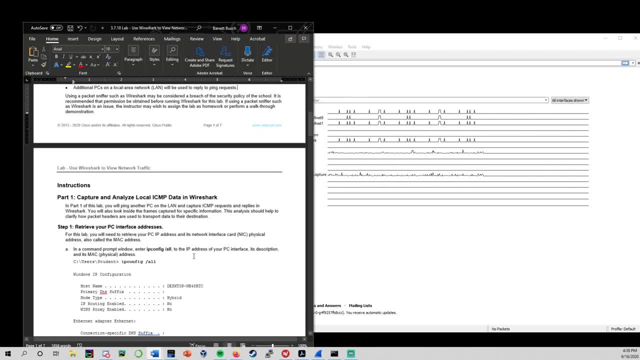 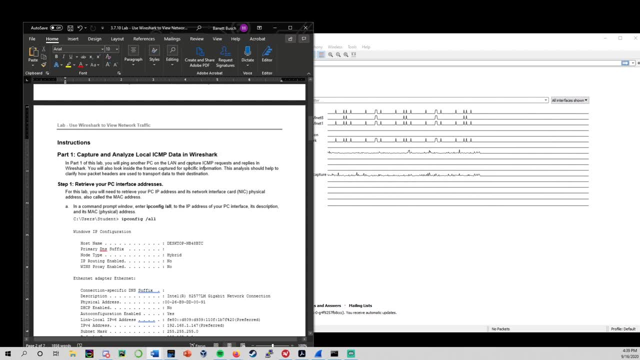 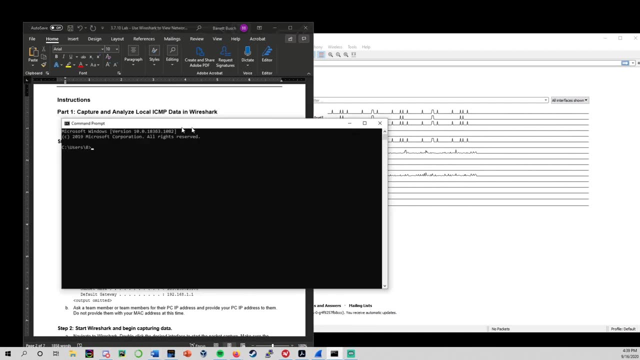 be the easiest option, So in part one we will. We'll capture and analyze local ICNP data in Wireshark. So first things first we need to figure out, okay, what is your local IP address or your private IP address. 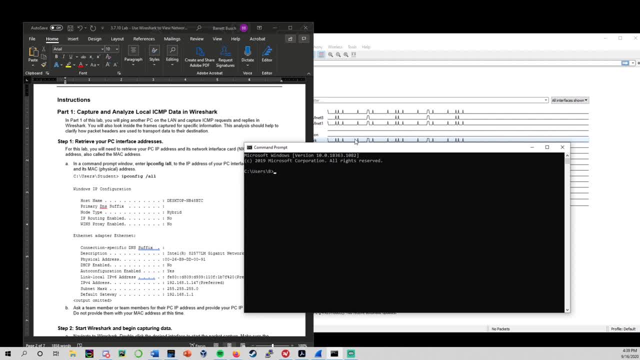 And as you work on this, don't worry, Even if you share those documents, this information with others, this is all internal, So you're not. You probably hear the phrase: don't let anybody, Don't let anybody ever know your IP address, and I obviously wouldn't be recording this. 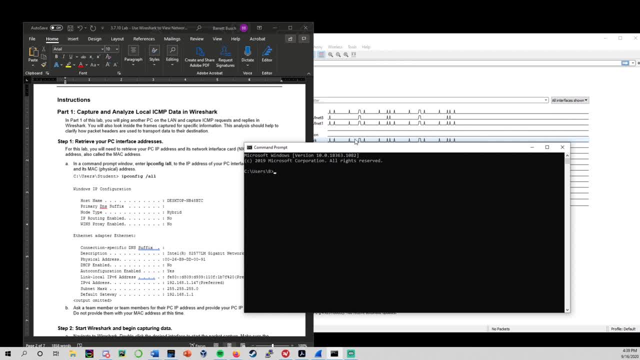 if it was bad, but your internal IP addresses don't relate to how other people can connect to you. That would be if it's your public IP address, which is your public-facing end of your router. That is something that you don't want to share, but in this case we'll be working with only. 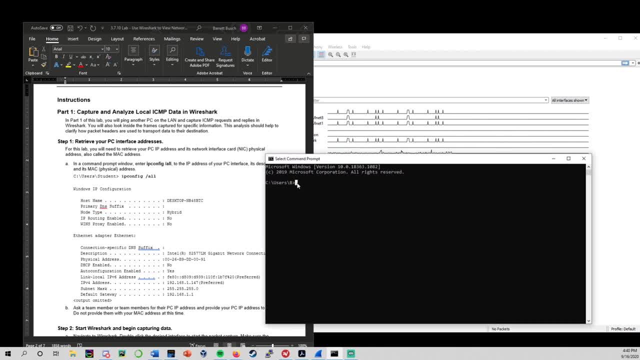 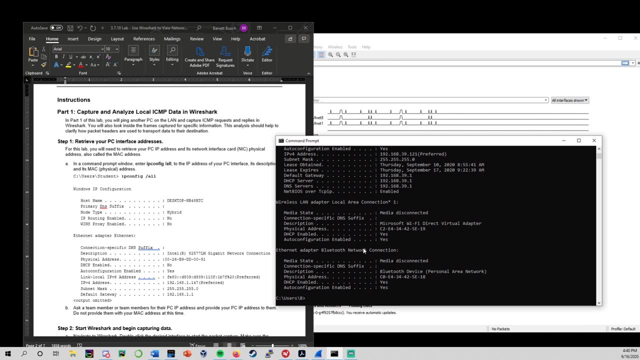 internal IP addresses. We're not going to be doing IPs for our own private network. So what we want to do, we could run ipconfig and then forward, slash all, and this is a tool that we could use to gather all of the details of our internal network. 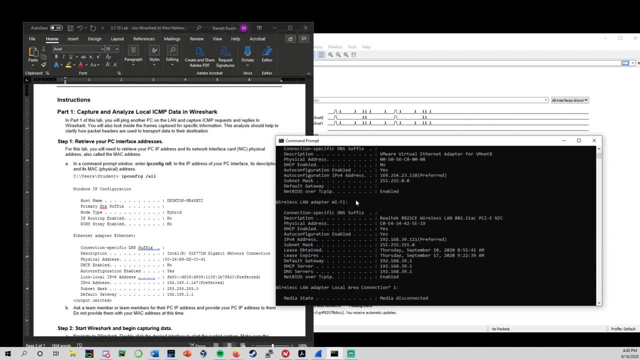 And so me personally- I'm going to be looking at my wireless adapter, because this is my internal adapter, because this PC that I'm running on is connected to the wireless network. You may see something different if you're plugged into a cable. 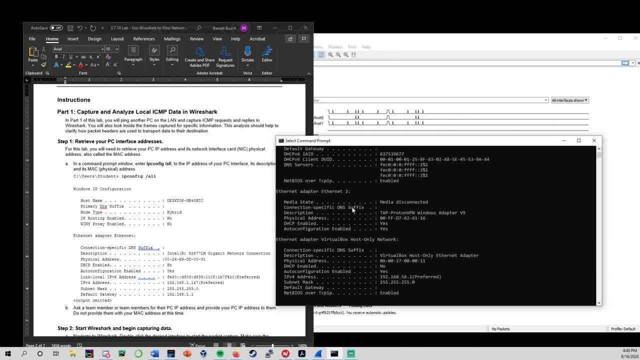 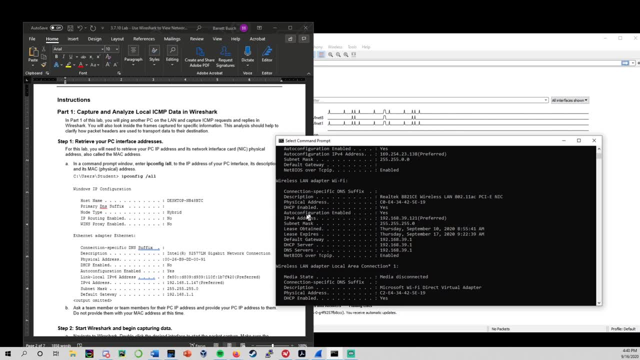 You'll see under probably Ethernet adapter here somewhere, But also I think a lot of you will probably also be working on your wireless as well. So what I see here? I have my IPv4 address right here, and then I'm also going to take. 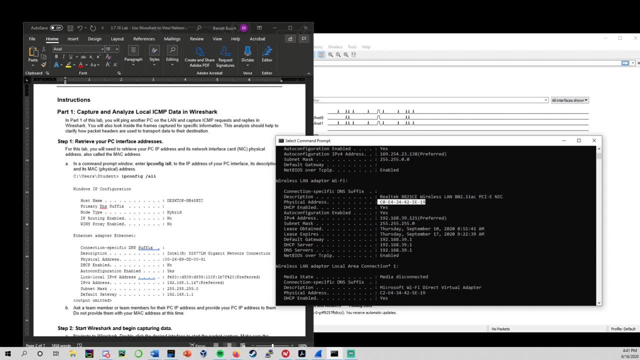 note of my physical address or my mobile address. Okay, My MAC address And what I'll do, and I would recommend you do it as well. I'm just going to pull up Notepad And I'm going to note these down. 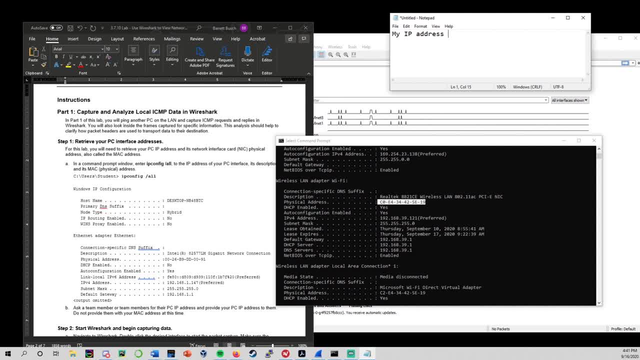 So I'm going to say, okay, my IP address is 192.168.39.121.. So now this 192 address, this is a private IP address. Other private IP addresses you may see begin with 10, and others also begin with 172. 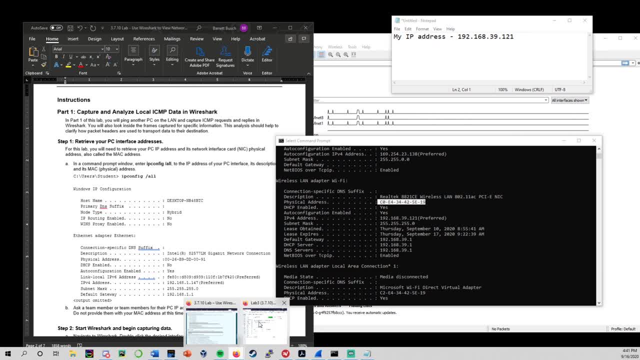 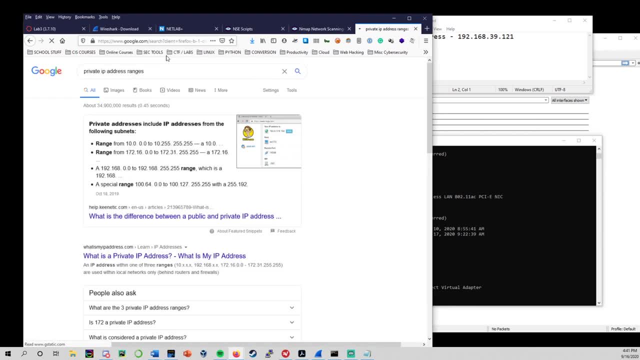 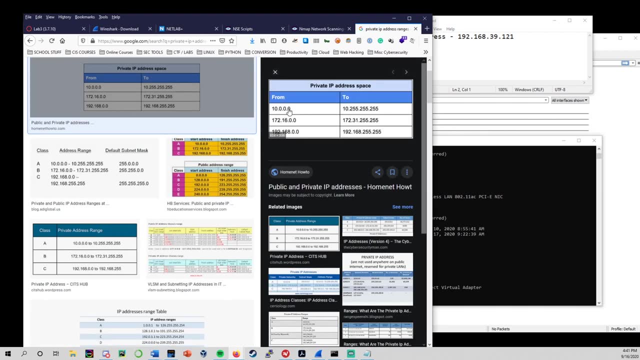 And even if you hold up, you can Google private IP address ranges if you ever forget this, and usually there's some pretty handy images you could pull up So you could see anything from 10 to 10.255.255.255. 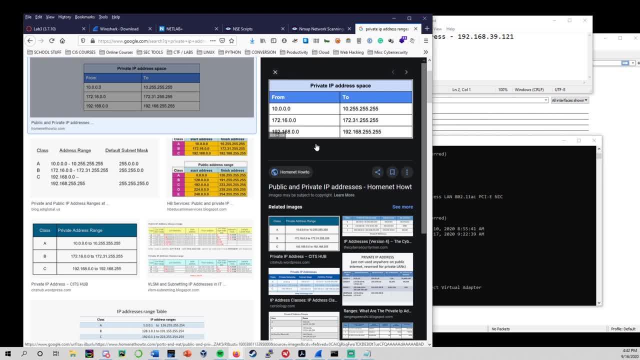 Okay, Okay, Okay, That's a private address space. Now, 172,- it's only going from 172.16 to 172.31, is a private IP address space, and then 192.168 is a private address space, and you can see that that is the one that I am in here. 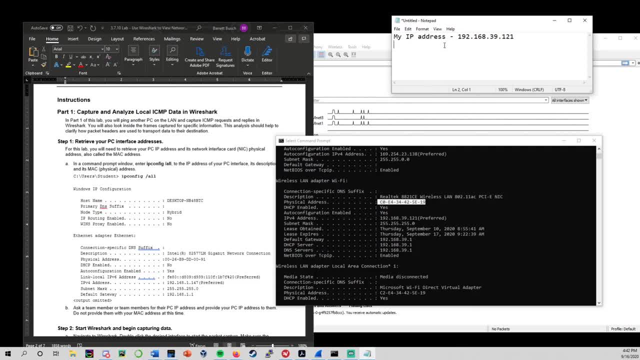 Now I'm also going to note: Okay, Okay, Okay, Now I'm just going to go in for my MAC address, C0E431.. And then also I mentioned how we're going to be pinging the default gateway. You can find that information right here as well. 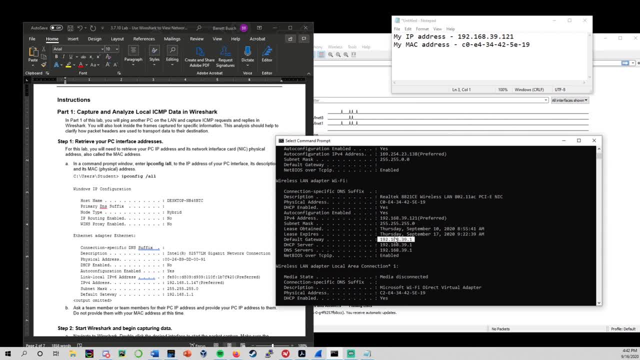 And you've probably heard me mention before that the default gateway is always going to end with the host.0.1.. And this also is in the default gateway, Pretty much another way of saying your router. Okay, So we have that. Eventually we will get to finding the default gateway MAC address. 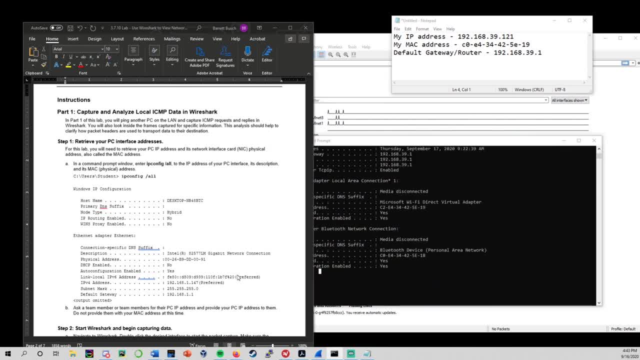 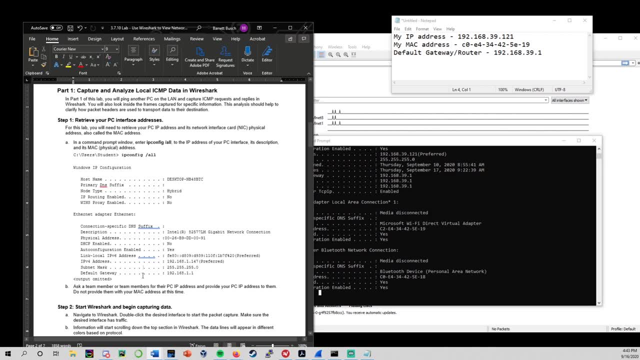 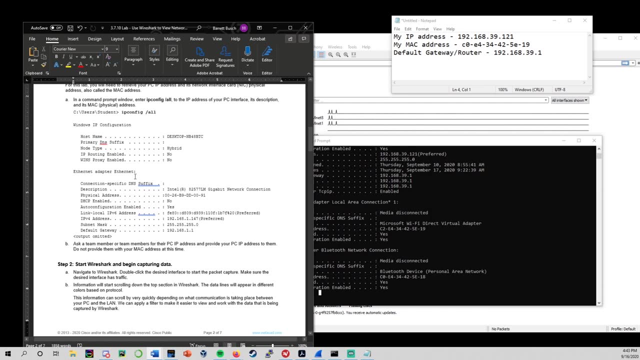 We'll come to that in just a little bit. So you could see that this information looks pretty similar to what's in the lab here. Obviously, this lab is different. It was scanned on a totally different machine, So your information is not going to look identical to what's in the lab document. 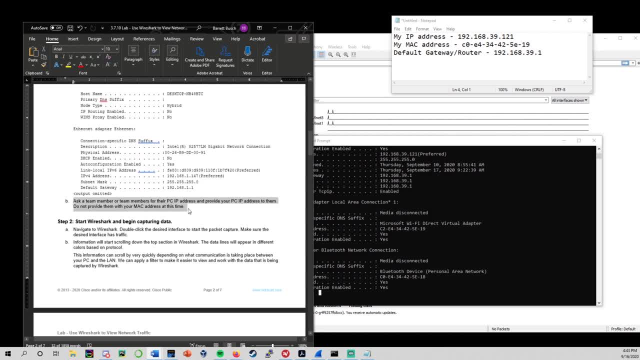 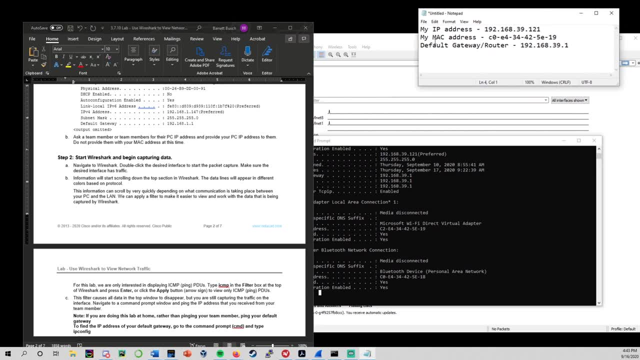 So, okay, ask a team member for their PCIP. We'll skip that at this time because we're going to be using the default gateway. Okay, So we want to navigate to Wireshark And straight away from this opening screen. 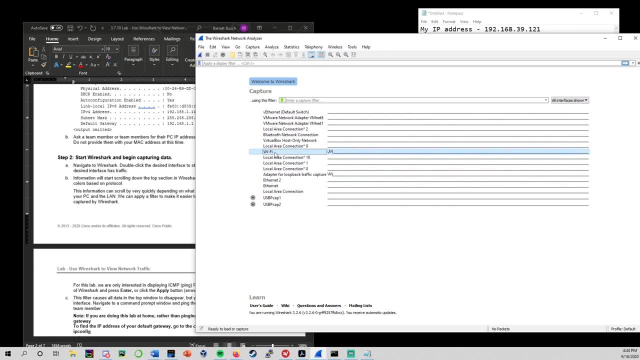 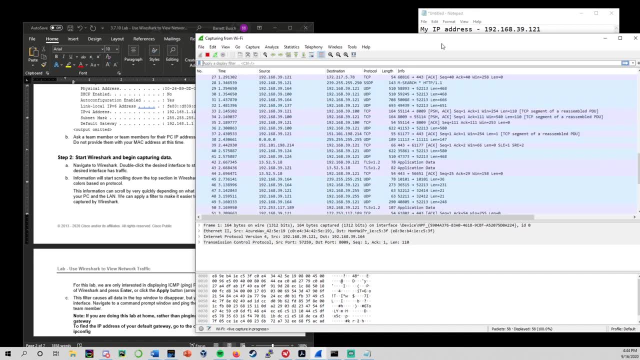 we want to select the interface, So I'm going to select the interface to capture. So I'm going to capture my Wi-Fi. I'll just double-click. You can see right away it's capturing a bunch of random packets that are happening. 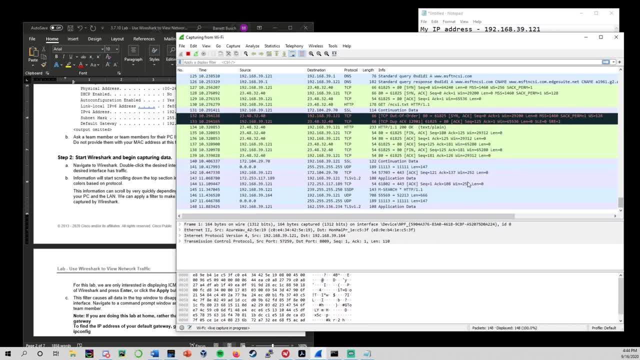 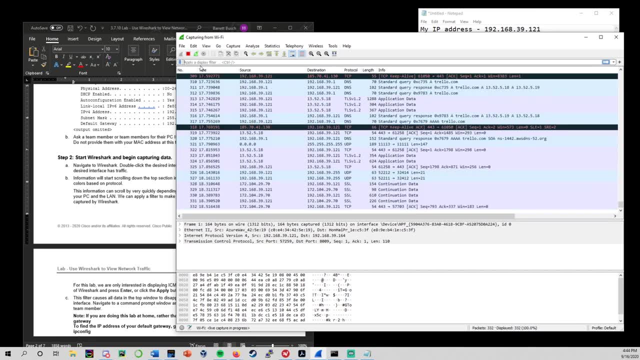 All you know, home networks have all sorts of information being passed around. So what I'm going to do first is come up to this display filter, And in this lab, all we're looking for is ICMP packets. So I'm going to type in ICMP in all lowercase: 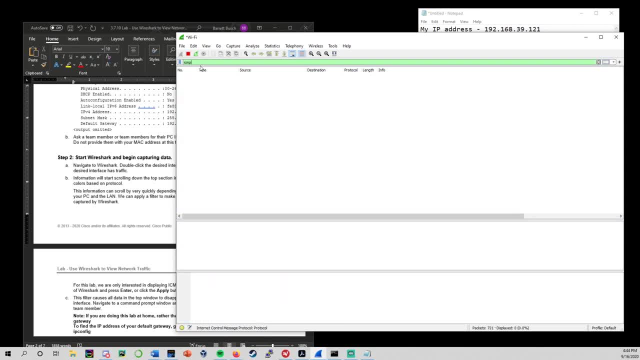 See the bar tag. Okay, The bar turned green. I'm going to press enter And you're going to say, okay, did that just delete everything? Well, no, because it's still doing the capture. We're just filtering the display. 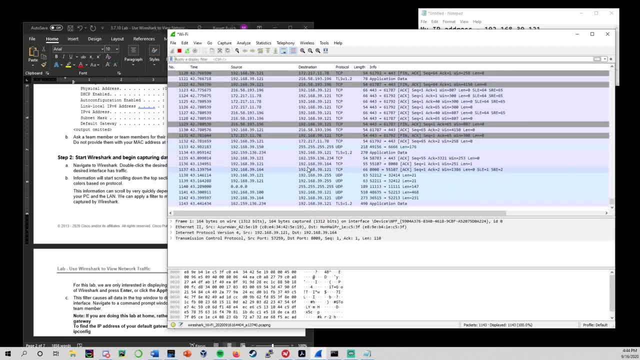 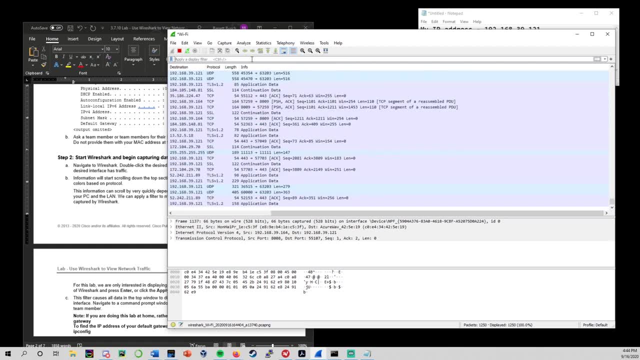 If I X'd out of this display filter, you see it's still capturing the background. We're currently at 1,200 packets right now, So I'm going to go ahead and refilter with ICMP. It's super important that it's all lowercase. 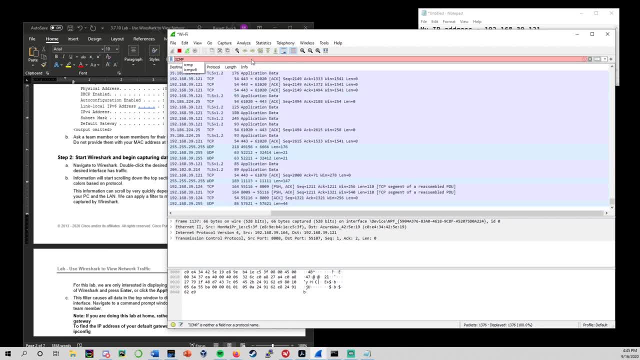 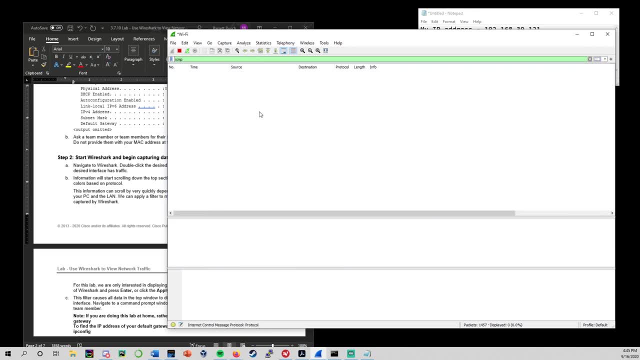 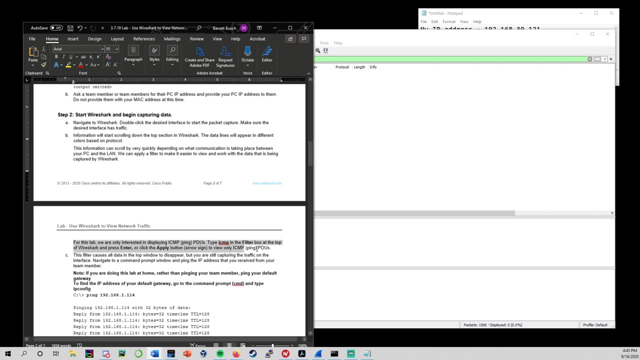 If you did uppercase ICMP, you see that bar is still red And it does not take the filter. So those always have to be lowercase. Okay, We have that filtered. You can see that in the B section here. the lab does go over that as well, typing in that filter. 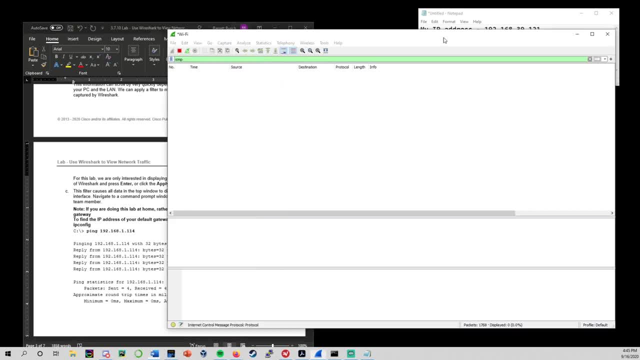 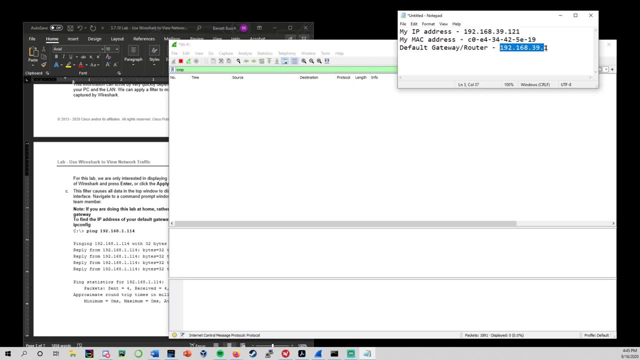 Great. So now we're at a place where we can go ahead and make our first ping request. So, remember, we're going to be pinging from our machine, We're going to ping our default gateway. So remember, your numbers will be different than these. 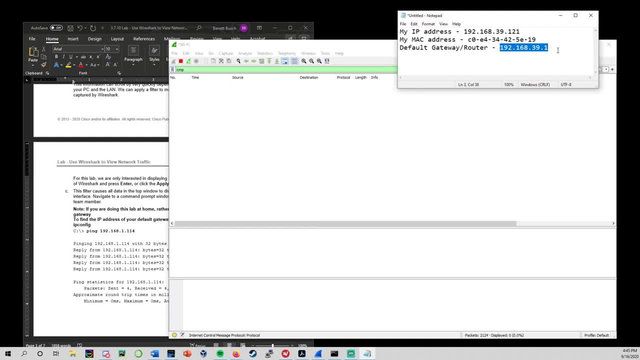 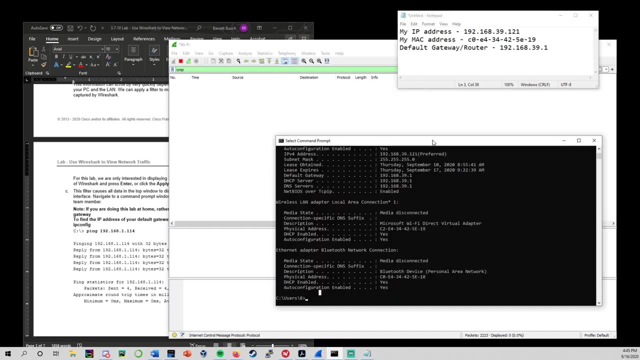 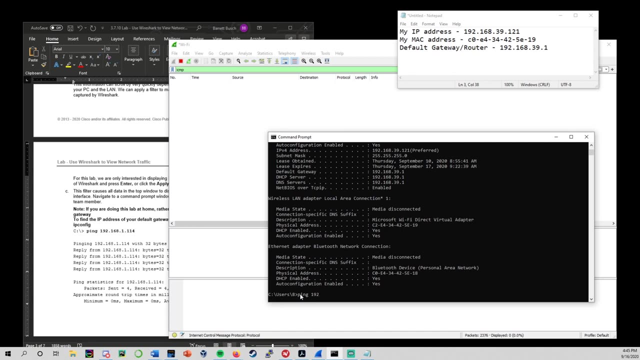 So don't ping what's on. you know my screen here. Make sure you ping from the information that you gathered about your own machine. So I'm going to come back to the command prompt. We'll just type in: ping 192.168.. 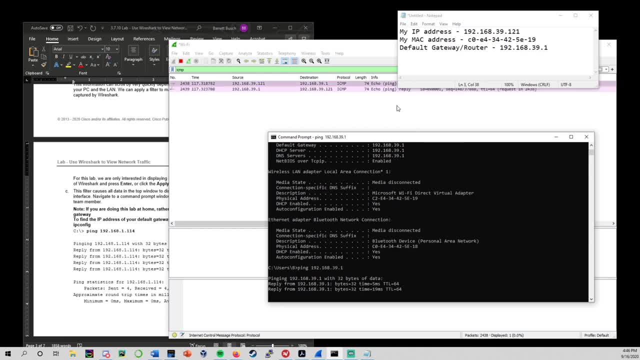 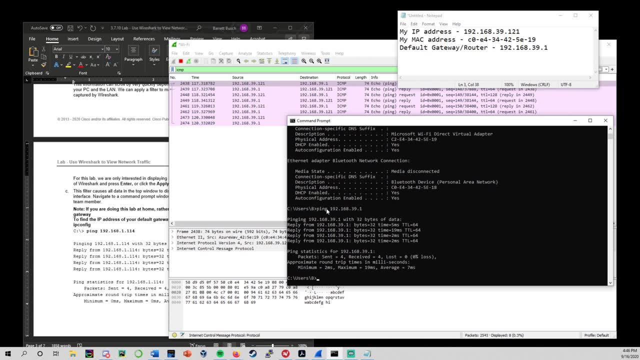 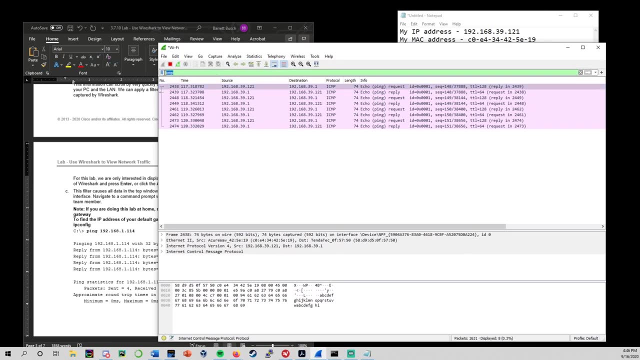 39.1.. Okay, So we see the pings going through here. Windows by default sends four ping requests, So I'll minimize this And now, because we had this filtered, we see all of these ICMP packets. So the very first. 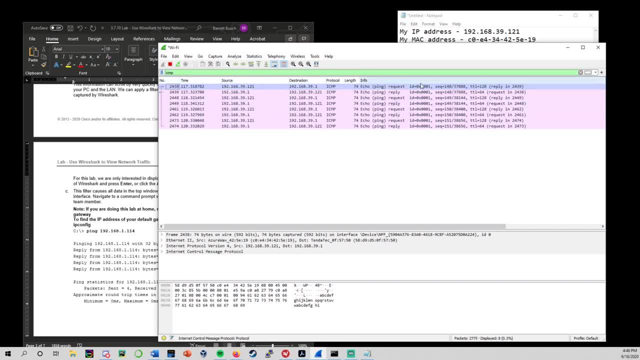 Well, let me break down what's happening in these different Wireshark columns here. So we have number And this is the packet number. So, as we mentioned before, we've been capturing packets for a while now, So we're already up to number, you know 2,438.. 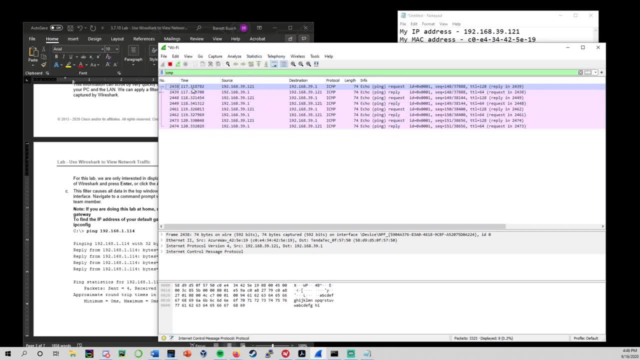 The time shows you the time that has passed. So we went from 117 to 120. So we could say that this ping took about three seconds. The very first packet, As we can imagine, that's the ping request. So it makes sense that the source IP comes from my IP address. 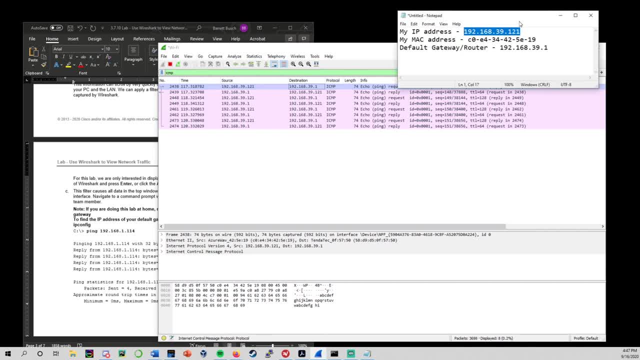 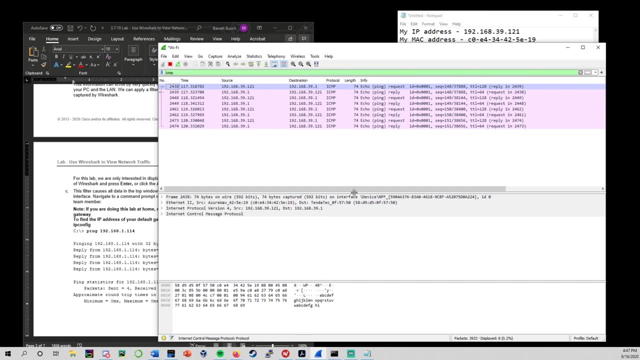 And the destination, the .1, is, of course, the default gateway. We see that these are listed under the ICMP protocol. Great So, And also you could see if you look in this middle window here you could drop down the Ethernet 2 frame. 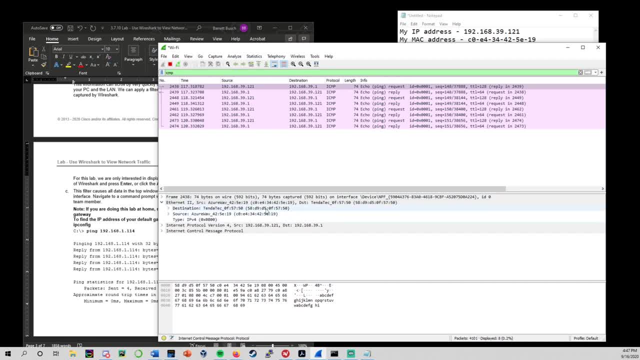 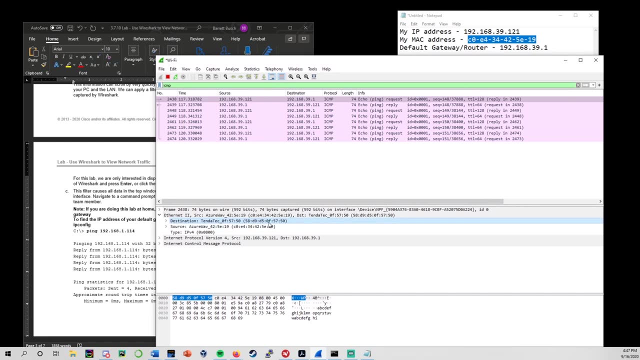 That's going to give you information about the source and destination MAC address. So the source, of course, is my PC. That matches that. And now right here we can say: okay, this, We just determined what the MAC address is for the router. 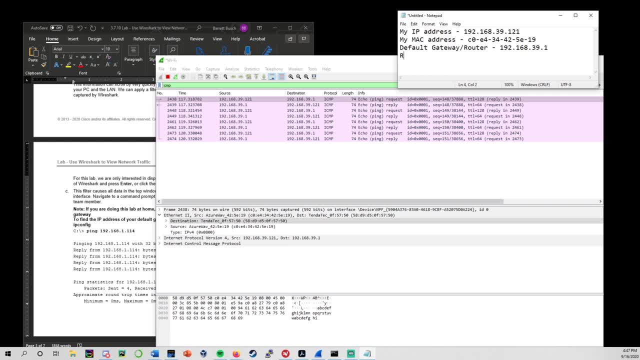 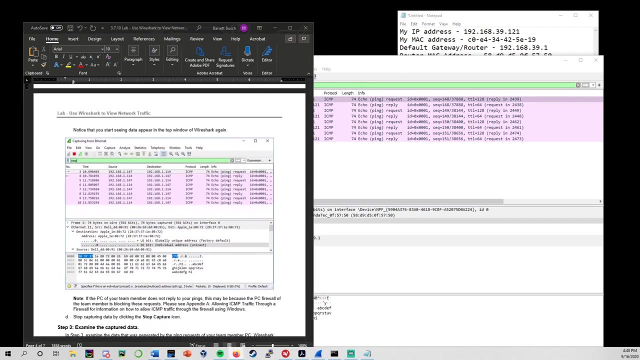 So I'm going to actually note that down as well. Router MAC address. That'll definitely come in handy when we're analyzing some other packets. Okay, so back to the lab. We did that first ping. Okay, we took a look at that information. 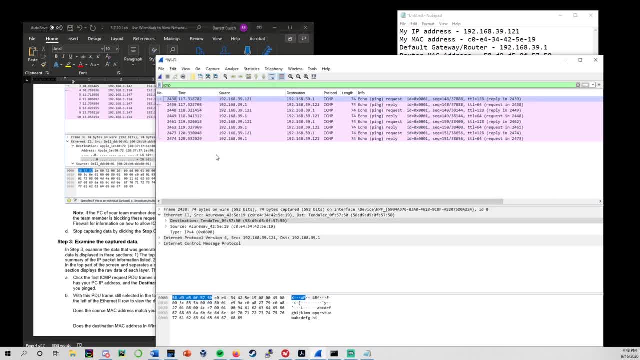 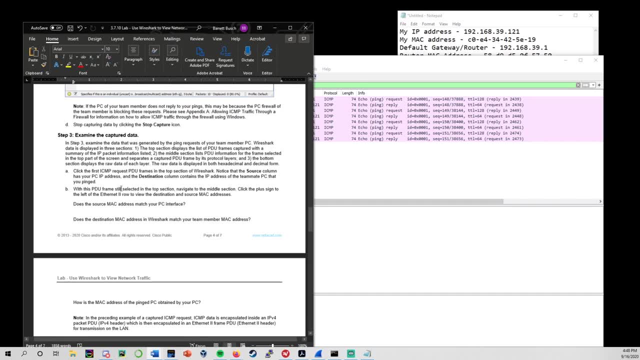 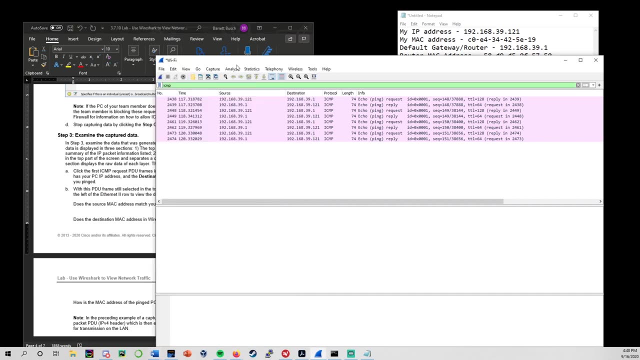 And also, I think at this point we can go ahead and stop this particular capture And we'll just be examining it. So we get down to the questions here. Does the source MAC address match the PC interface? Yes, We confirm that the source right here matches. 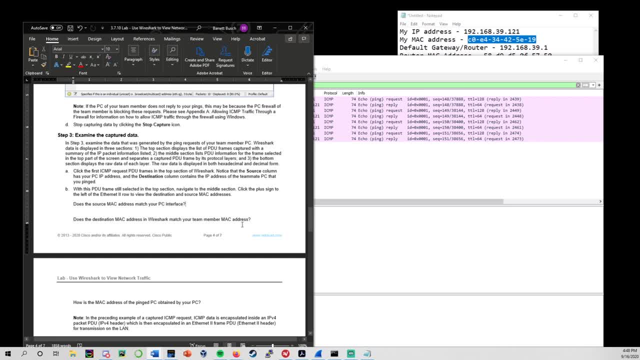 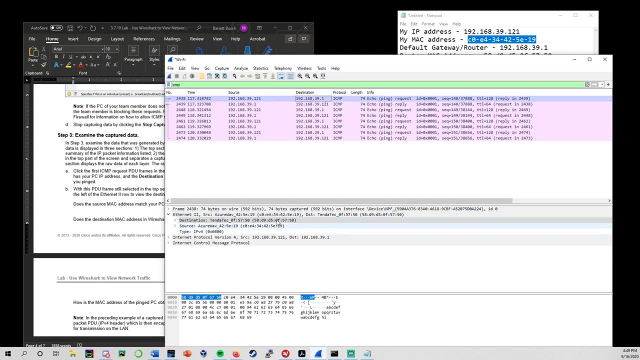 Does the destination MAC address in Wireshark match your team member MAC address? Or in this case it's our router? So that's actually a good question, Because you could say: well, how do we know for sure? At this point we're trusting that Wireshark is reading that correctly. 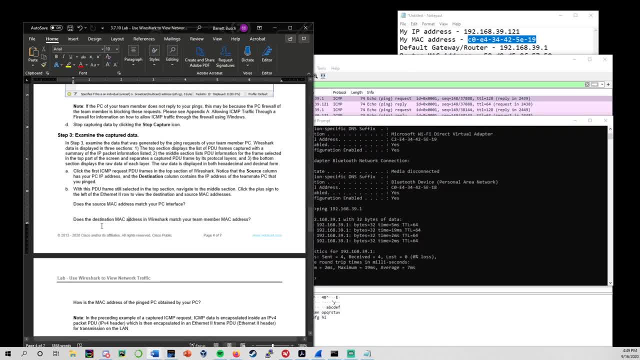 But what we could do. This kind of takes into Consideration. this third question here: How is the MAC address of the pinged PC obtained by your PC? Well, this is done by what's called an ARP request or address resolution protocol. 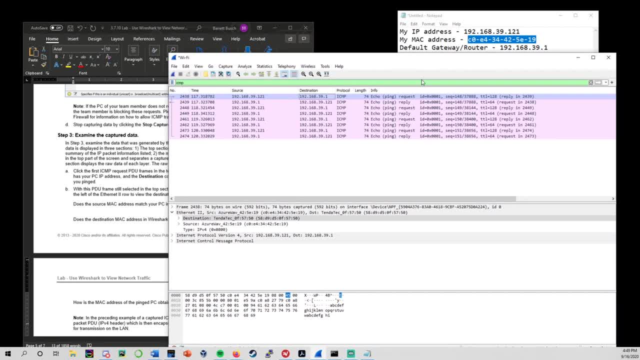 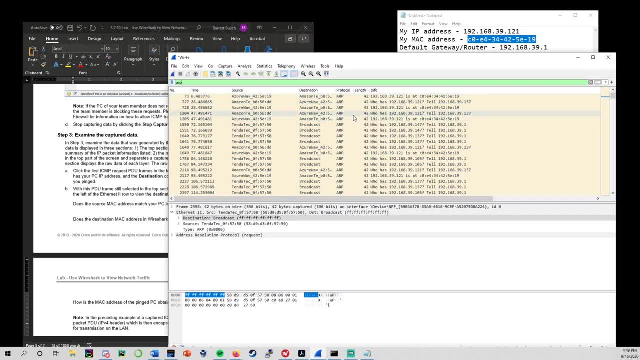 So I could actually change this display filter and search for ARP. So you see all these ARP requests here. What this does? it sends out a broadcast message. You see that under destination here broadcast, And it's essentially saying: okay, who has such and such IP address? 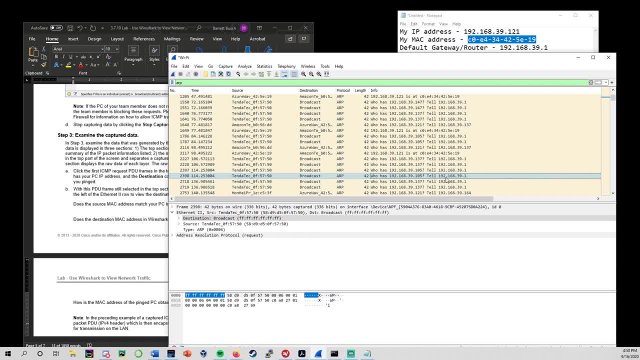 And you see, in this case it's saying TEL 192.168.39.1.. And we actually know that to be the router, So which totally makes sense because you know your network has a bunch of different machines. 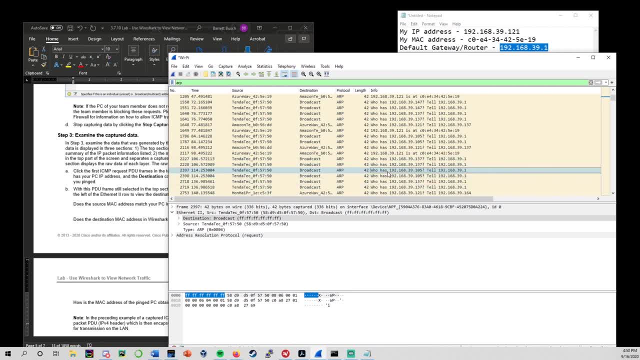 And it's always going to have to go through the router, You know, especially if it's connecting to the internet. So what that router will be doing, it'll be creating a table of MAC addresses and how they relate to the IP addresses that make these kind of requests. 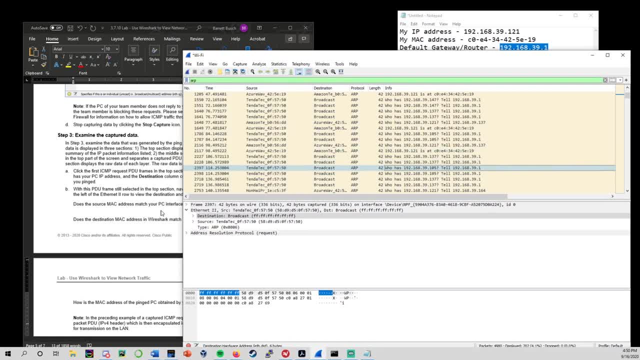 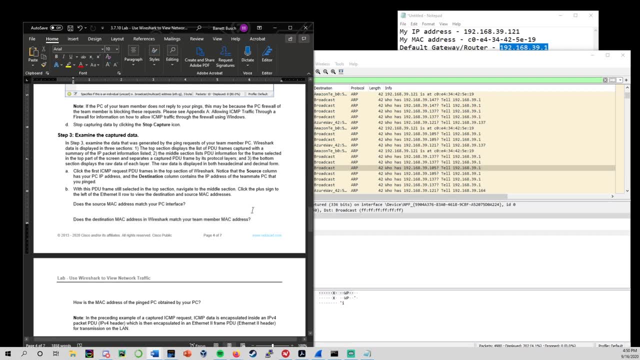 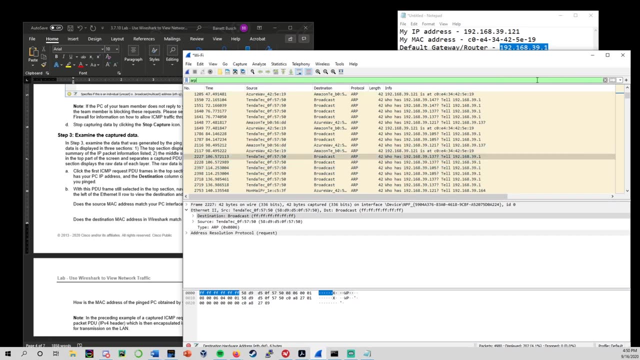 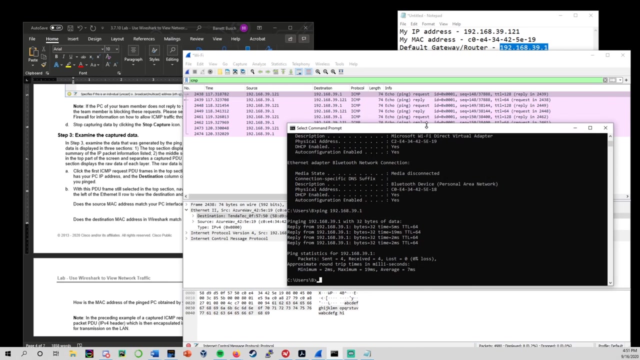 So that's how, through this ARP request, that's how we come to find the MAC addresses of particular machines. So what we could do to kind of verify. I'm going to change this back to ICMP filter. This is kind of a little bit outside of the lab. 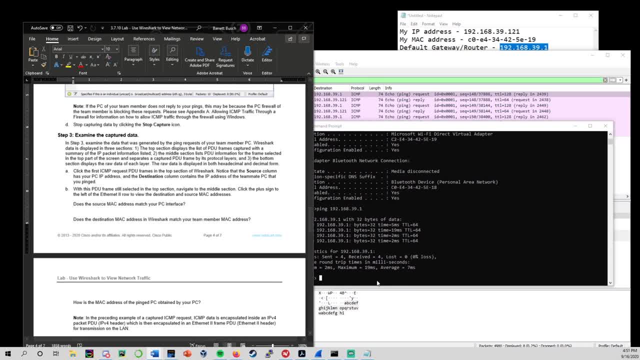 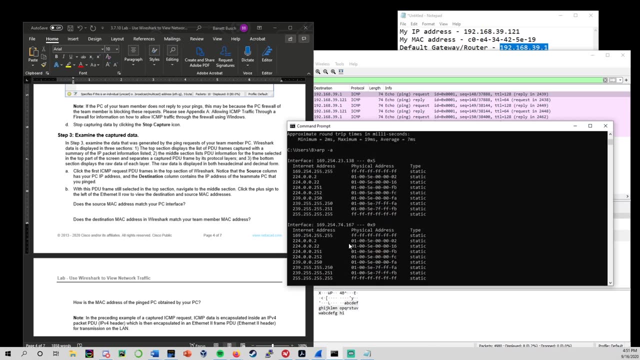 I don't believe the lab goes over this, But what I would essentially do is run the ARP command in the Windows command line and do "-a", And this is actually going to show you some of the ARP tables that have already been populated on my machine. 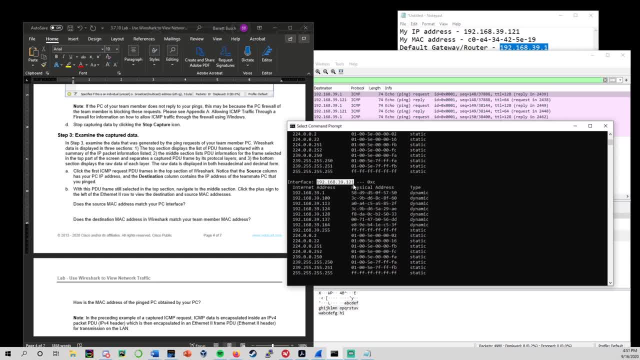 And so I'm finding the interface for my IP address And essentially what you want to look for: find the IP address of the router. We see that right here, And so I can actually reconfirm the physical address or MAC address of the router. 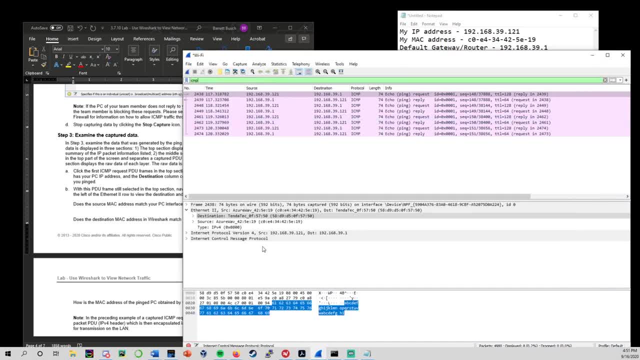 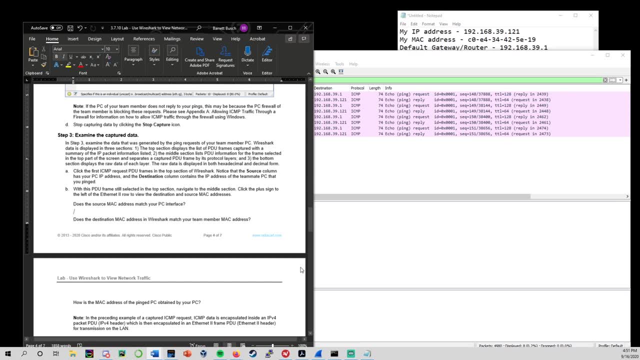 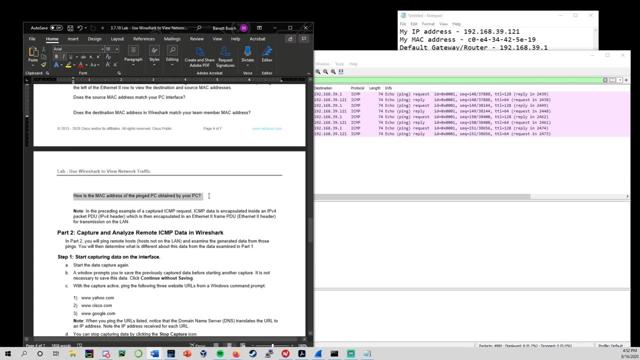 So that looks like that was correct, So we can confirm that what we see here in Wireshark was indeed that MAC address. Great, So yeah. So, once again, how is the MAC address of the ping PC obtained by your PC? Very simply, the MAC address is obtained through an ARP request. 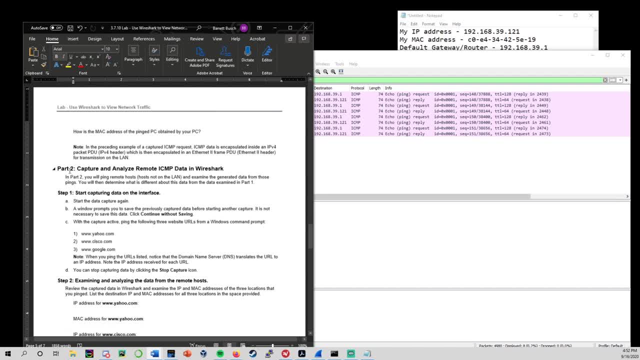 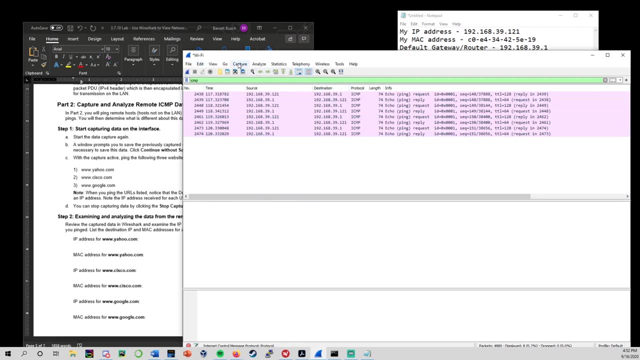 Okay, So we will move on to the second part of the lab: capturing and analyzing remote ICMP data. So this is where we're going to be pinging outside websites, And so I've already stopped the capture, So we're going to create a new one. 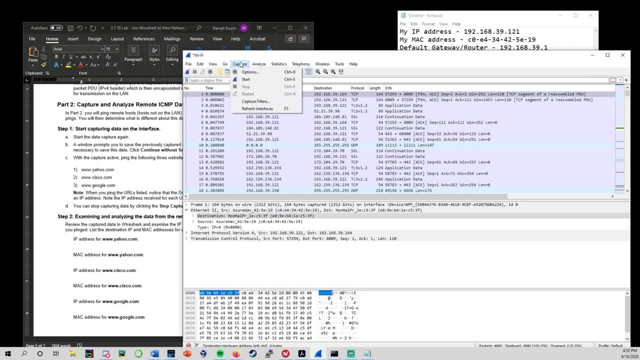 Get out of there. Let's go to Caption Or- I'm sorry, sorry- Capture And then just start And you can say: continue without saving. You don't need to necessarily save that PCOP file for anything. Okay, So you can see it started a new, fresh, capture. 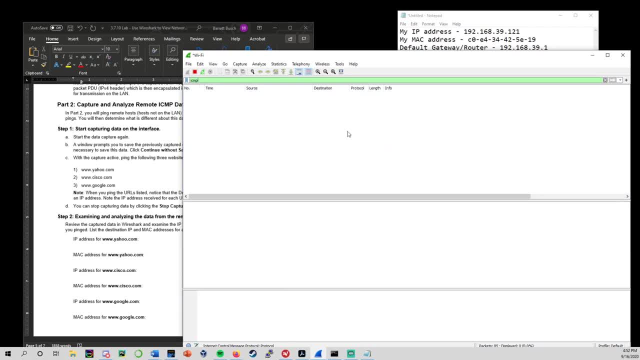 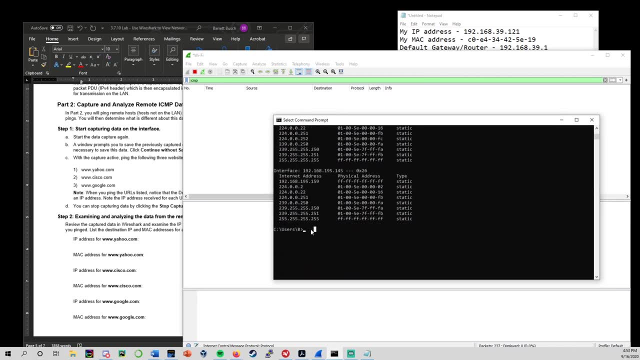 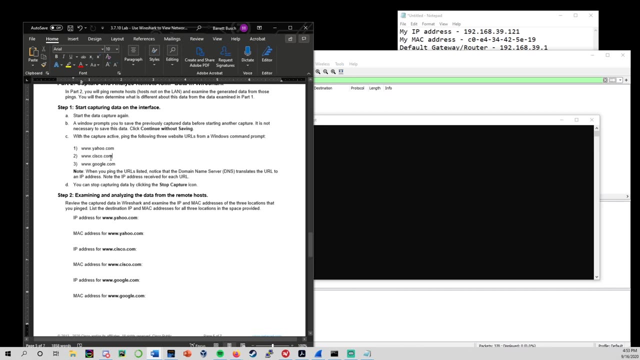 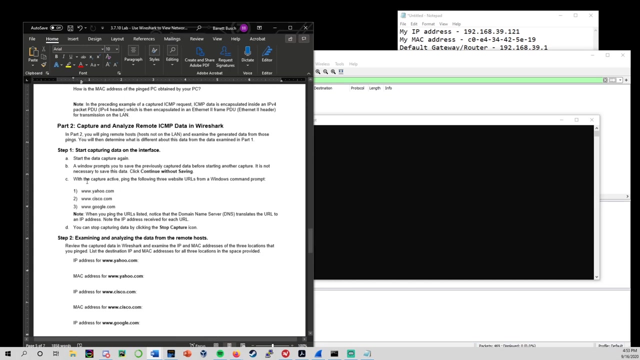 I'm going to go ahead and filter by ICMP again And I will pull up the command prompt again. Just go ahead and type CLS to clear the screen out. Okay, So review the captured data. Okay, Now I'm jumping ahead of myself here. 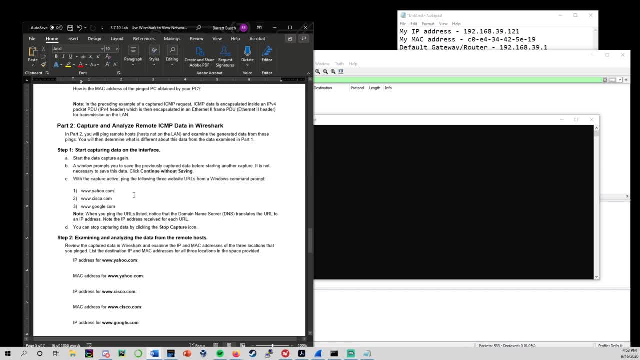 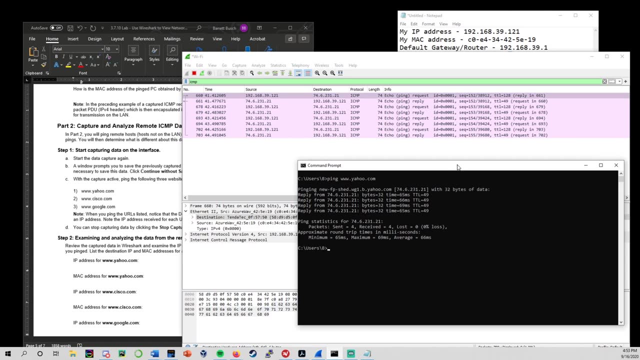 Okay, So we just want to ping these three websites. Ping wwwyahoocom: You could already see that happening in the background here, So you could potentially ping these all at once, or you could take them one at a time. I think I'm going to take them one at a time. 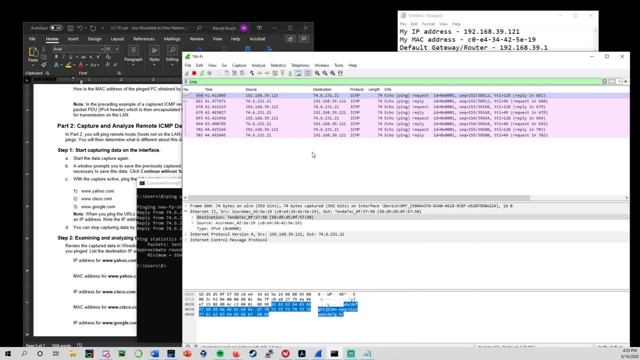 just so we can look at each chunk together. So We know that our IP address is this: dot 121.. So that makes sense. That's the first packet here. the source And the destination is this: 74.6.231.21.. 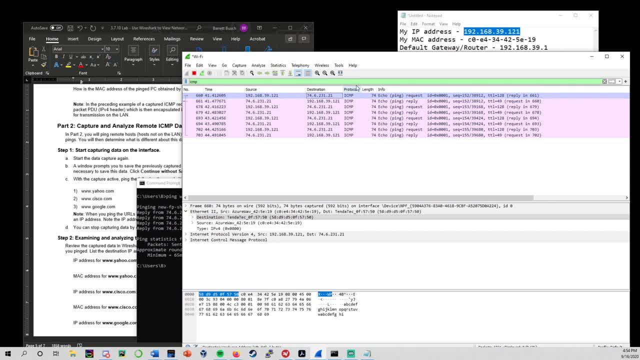 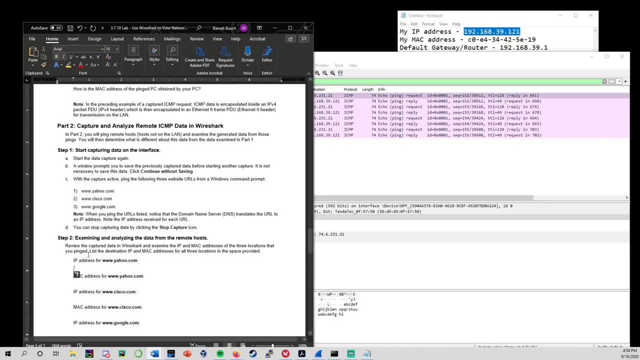 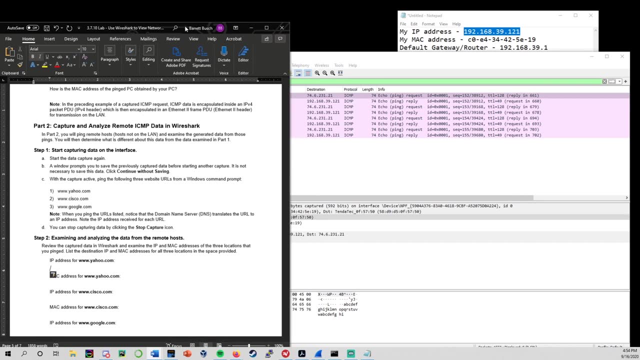 Now this is a public IP address, And so this is the IP for yahoocom. So in your lab you could just enter that in. I usually like to choose a red font: 74.6.231.21.. And then it's going to ask. 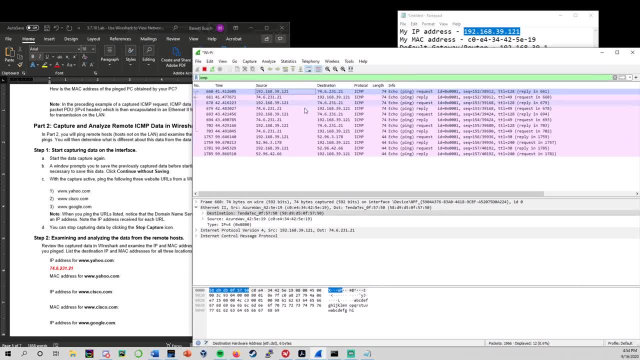 well, what is the MAC address for that? So this is kind of a trick question because, as we kind of talked about going over the sample quiz as well, if you are pinging a remote system or something external out of your own network, 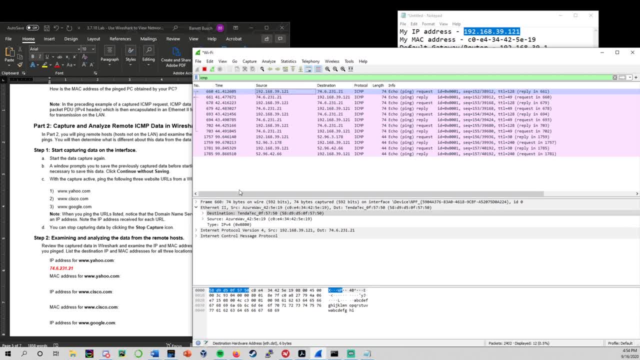 out of your local area network, you're not going to receive back the MAC address of that outside machine. What you will receive back is the MAC address of your router. So you know the answer to this question and you could see this in the destination. 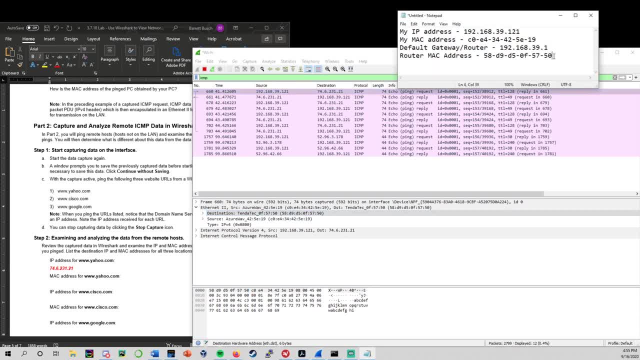 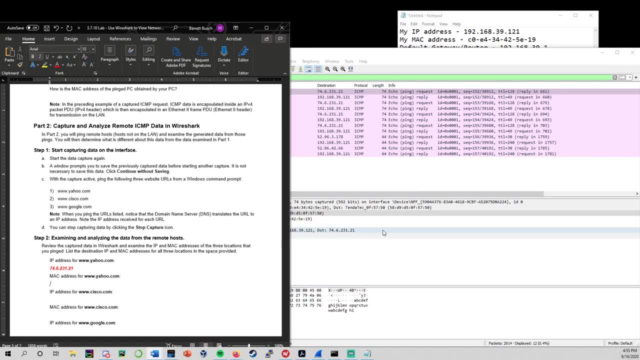 the MAC address here. it is the same as her router, Because you know that information you requested from yahoocom, it comes back to you through your physical router. So you know you could use this as the answer And I would. whoops. 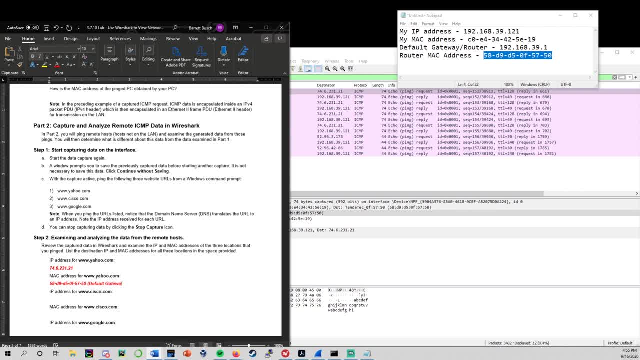 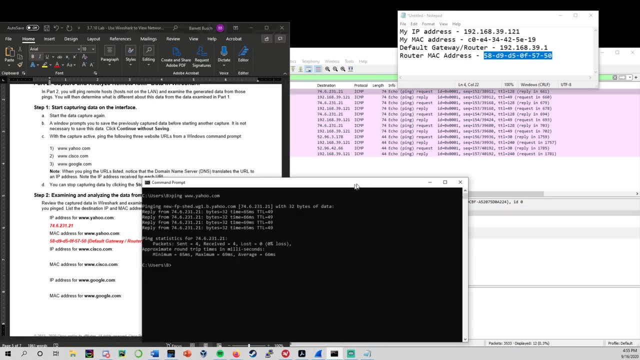 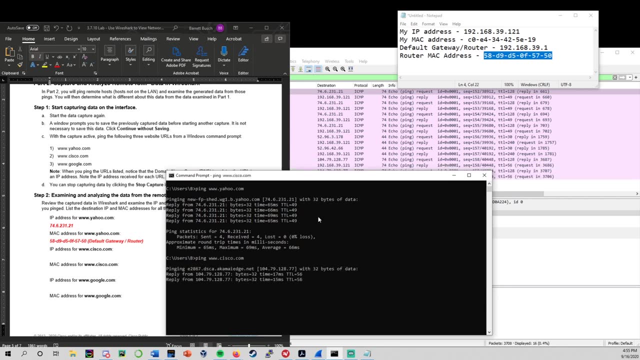 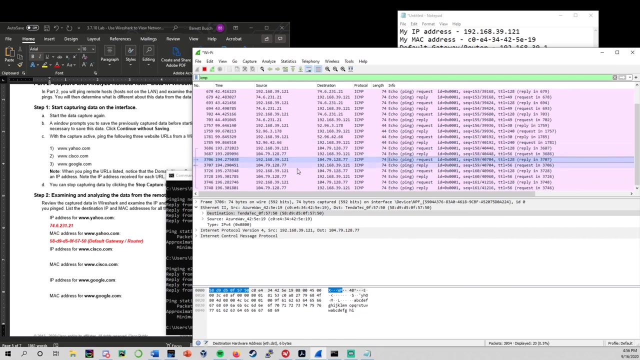 And I would probably just make a note: default gateway router. Then we move on. Now we go to ciscocom, So we'll do ping wwwciscocom. You see those being captured here. It's interesting. I actually have a ping request. 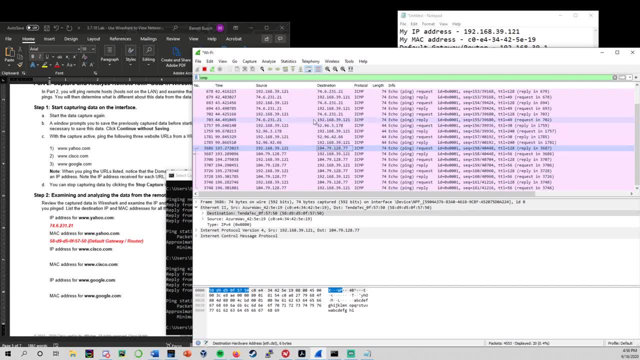 that popped up here that I don't believe I myself initiated, So I'm actually going to have to take a look into that. So ignore these ones right here. What we're looking at is this new bunch here, So we know that. 192.168.39.121. 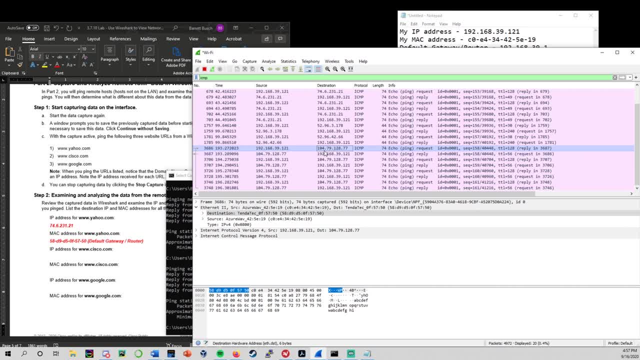 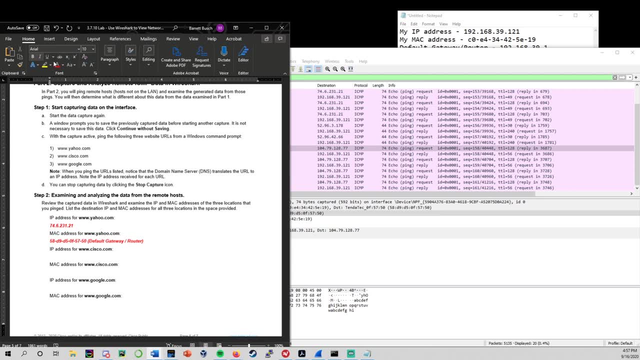 is my internal IP. So we're looking at 104.79.128.77 as the cisco address, So I would just go ahead and enter that in here: 104.. And so what is the MAC address for ciscocom? 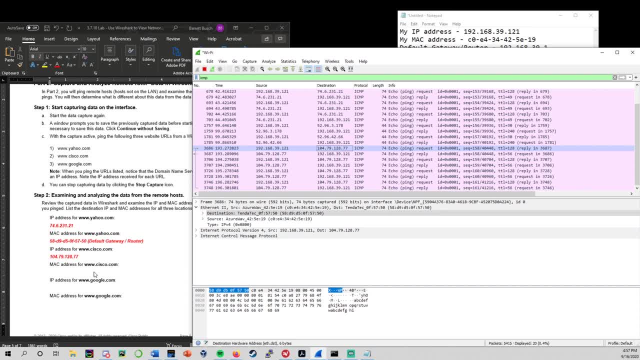 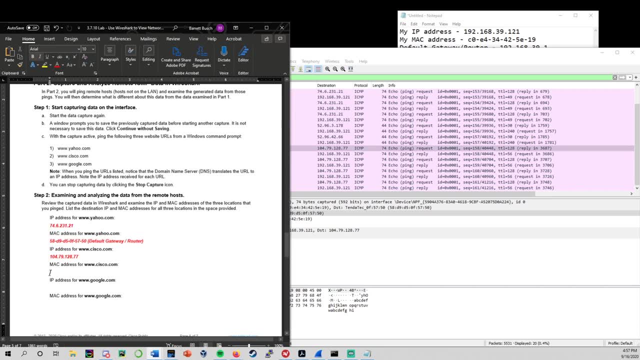 Well, trick question again. You know we can't. we don't know the MAC address of that cisco server or website, But what we get back is our router Or default gateway MAC address. So the answer for those you know are the same. 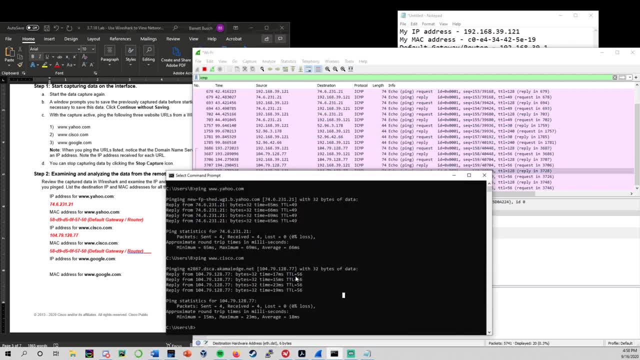 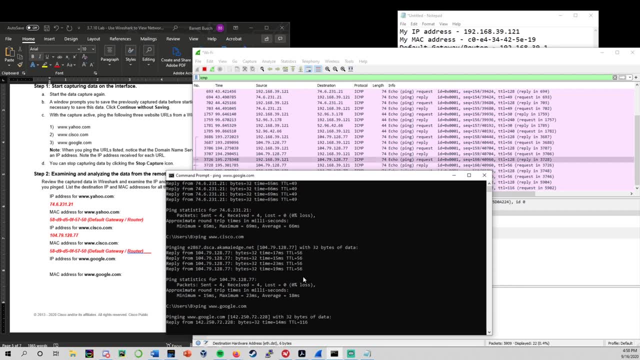 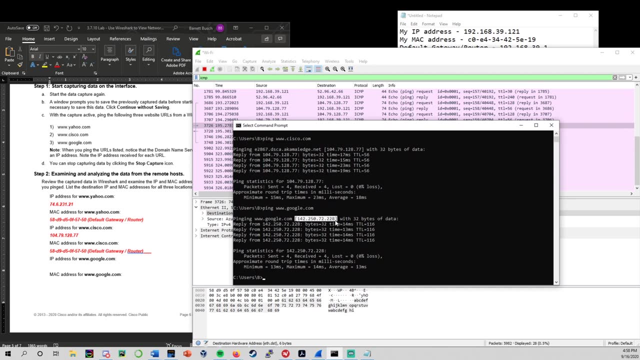 IP address of googlecom. Come back to command prompt Ping wwwgooglecom. You could see here it even gives you the IP address right here. Essentially, it's doing a DNS request. You're gaining that IP address straight away from there. 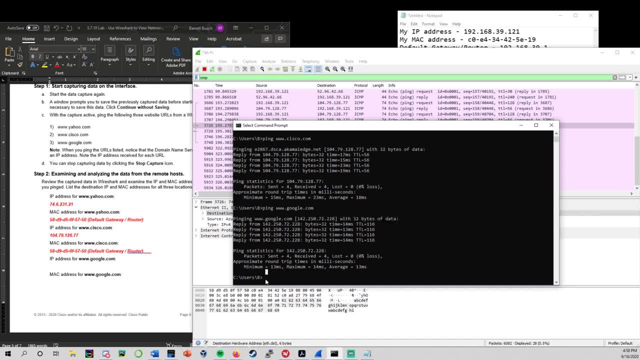 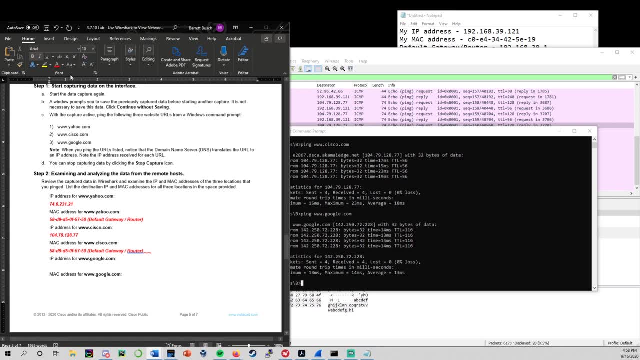 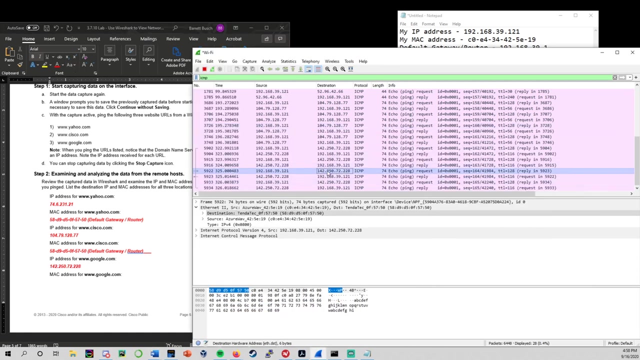 You're gaining that IP address straight away from this ping request or from the ping tool. You could even use that as reference And, of course, we could verify that in Wireshark Source IP from our internal destination to googlecom IP address. 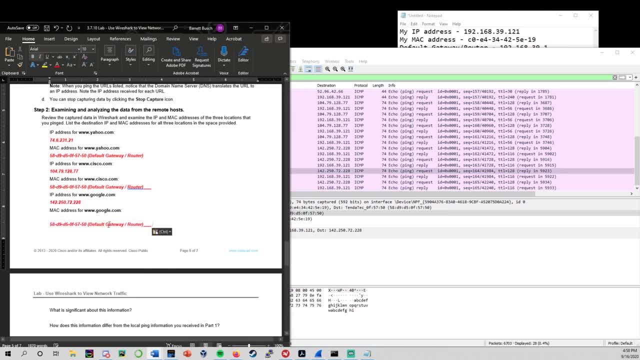 And, of course, MAC address. the answer is going to be the same: Because we're pinging an external site or host, we can't know their MAC address Only, it'll only come back as our default gateway. So what is significant about this information? 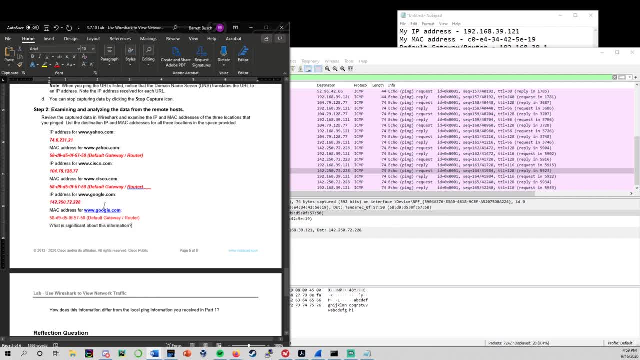 Well, essentially what we just said, you know the IP addresses being different here is not significant. That's expected. So I suppose what's significant is that MAC address results are all the same And of course, they all point to our default gateway. 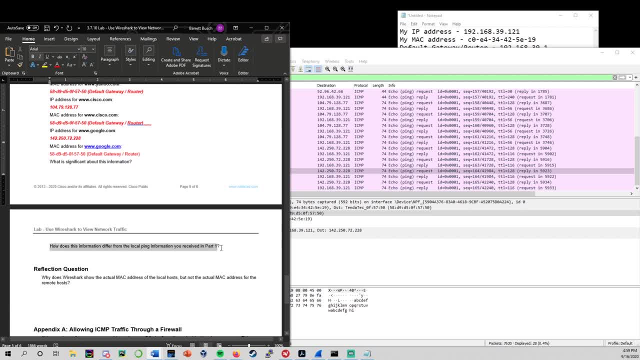 So how does this differ from the local ping information? You know, when you ping locally, that's going to return the MAC address of the PC's network interface card, right, It's going to return that physical address. But when you ping a remote host, 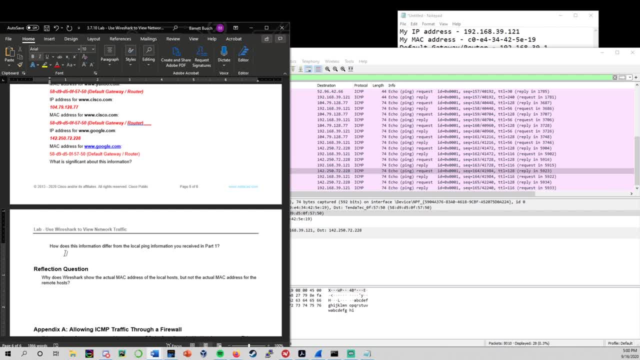 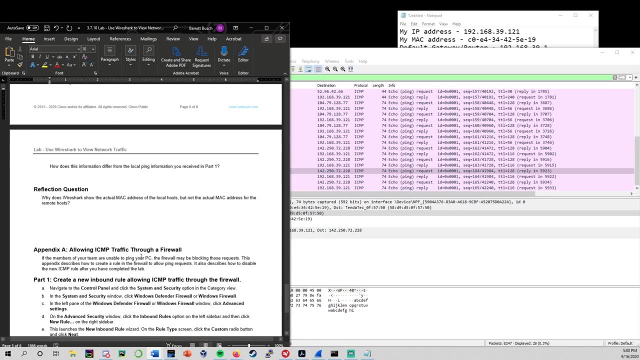 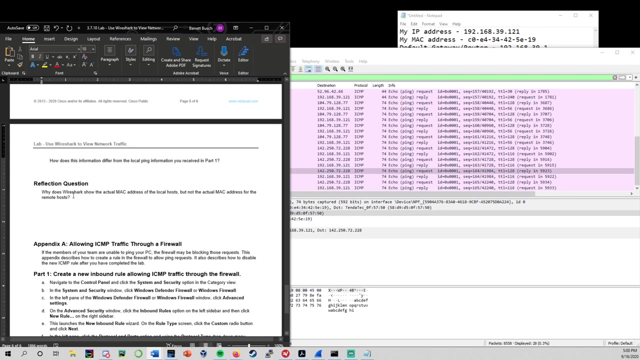 it's only going to return the MAC address of your default gateway or the, you know, the local area network interface. So that's essentially the responses for those questions. Okay, looks like we got to the end here, So the reflection question. 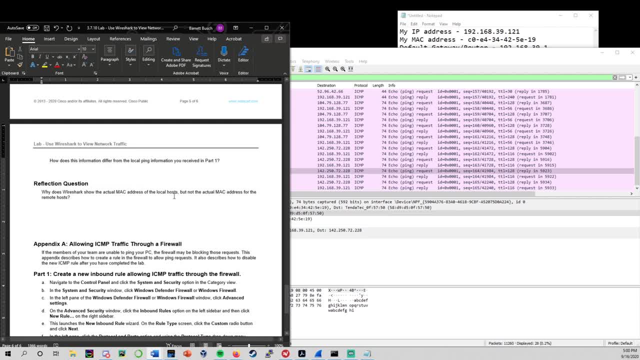 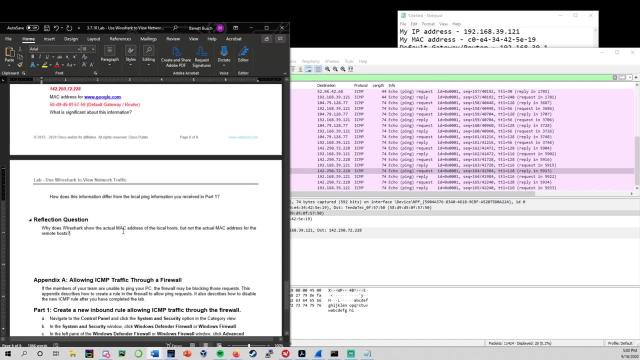 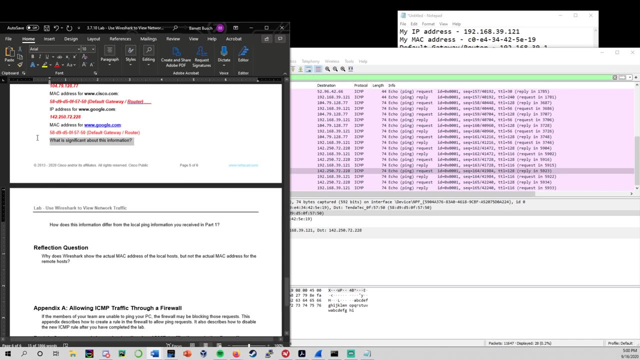 why does Wireshark show the actual MAC address of the local hosts but not the actual MAC address for the remote hosts? I mean, essentially that's what we, just what we just went over. It highly relates to these two questions here. 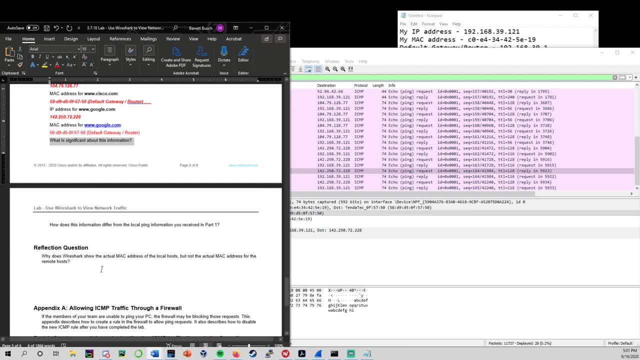 I'm going to leave you to kind of, you know, reflect on that question. You know, you can definitely find a lot of really nice information online about this as well, just by Googling. I encourage you to kind of like, look into this a little bit more. 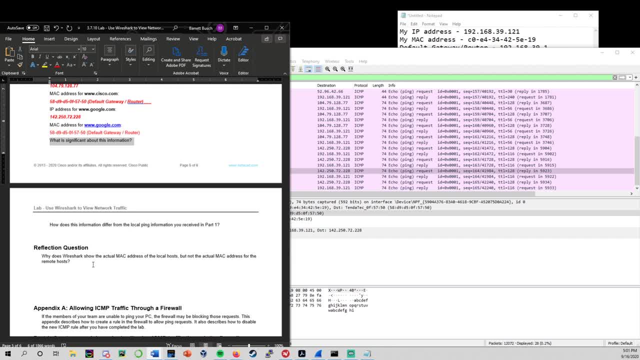 And you could also look into how this relates to the OSI layer model. also, What's the difference between layer two, information, and layer three? You know you have the data link layer where you know MAC addresses reside, those physical addresses. Then what's the difference between that? 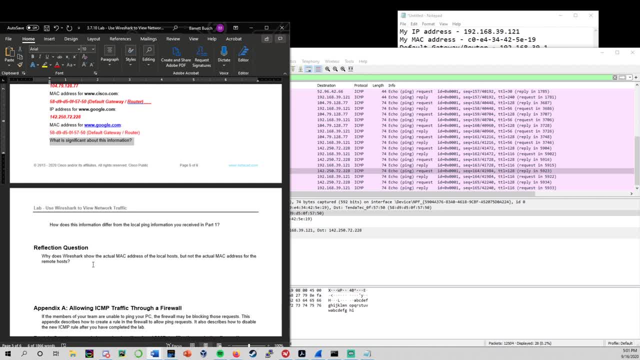 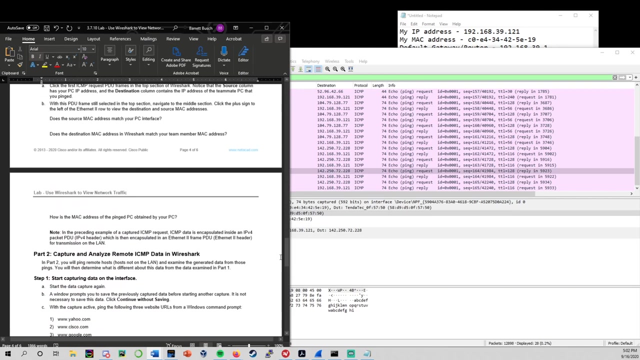 and layer three, the network layer, and using logical IP addresses. That is definitely something that you'll gain a much more deeper understanding of this question in your reflection on that So great. So that covers this lab. I hope you enjoyed it.